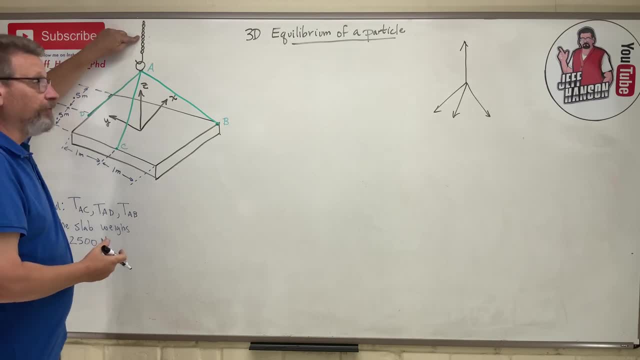 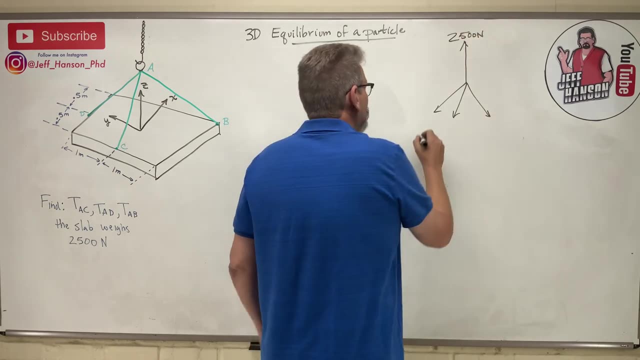 The force in that chain is 2,500 newtons. right, So that upward force there is 2,500 newtons, okay, And then this is T, what AD, The middle one is AC and this one's TAB. okay, So the way to solve. 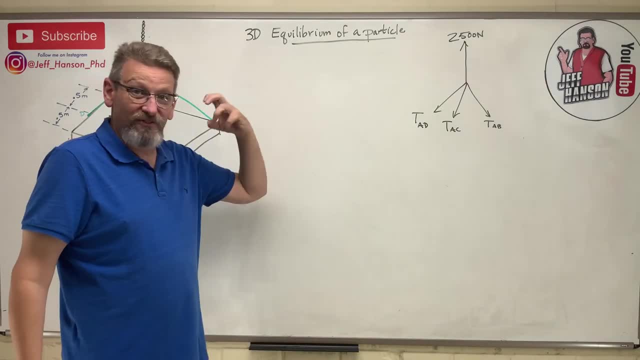 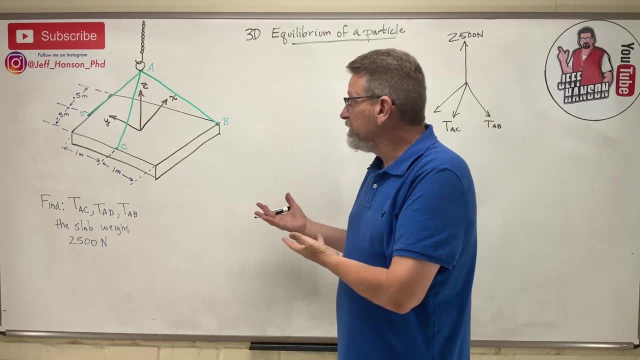 this problem is to. these are just vectors. they're 3D vectors. remember there's three ways: blue triangle, directional cosine, or with coordinates. what do we have here? We have coordinates. What did Dr Hansen not put on the board? One of the dimensions? 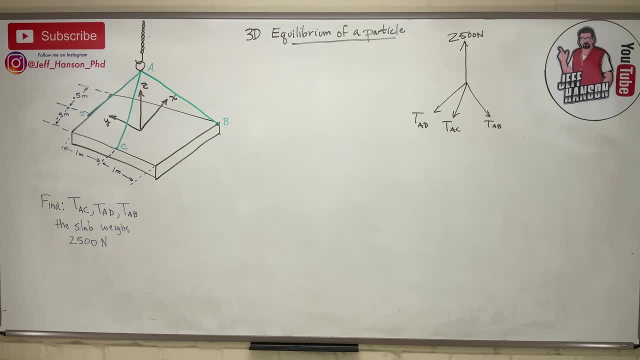 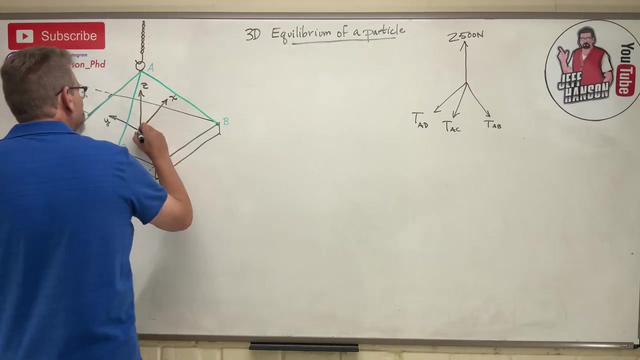 Well, right here. Okay. So let's make the dimension from the grace. Okay. So, let's make the dimension from the grace. So let's make the dimension from the grace, the top of the plate to the hook up here, two meters, okay. so this whole thing right here is. 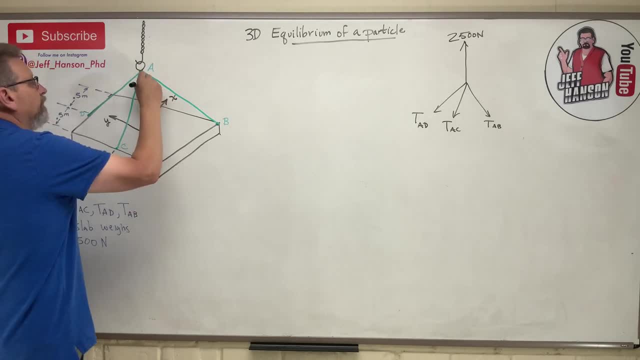 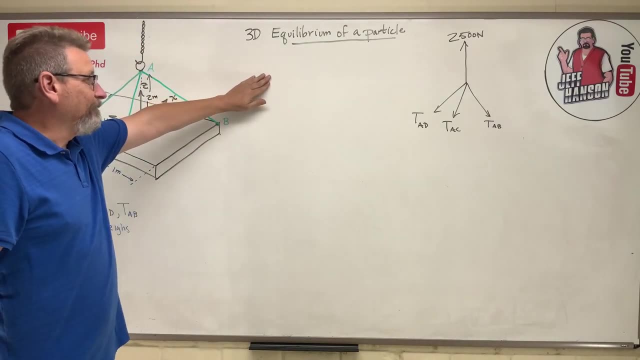 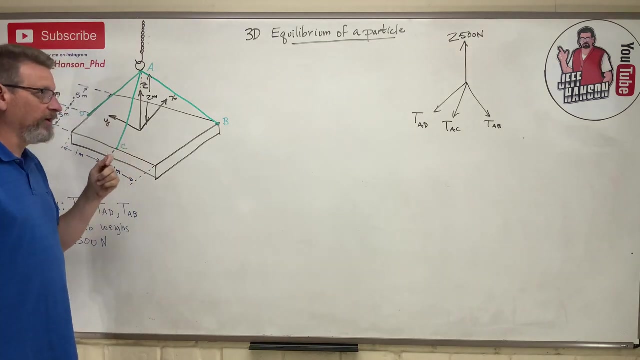 two meters from here to there. okay, there you go. that was, I left that off, 10 points off for me, okay. so here's what we got to do. we got to write these 3d vectors with lambda hat, right, because these are definitely with coordinates, and so what would lambda happen? if you remember, is f vector f. 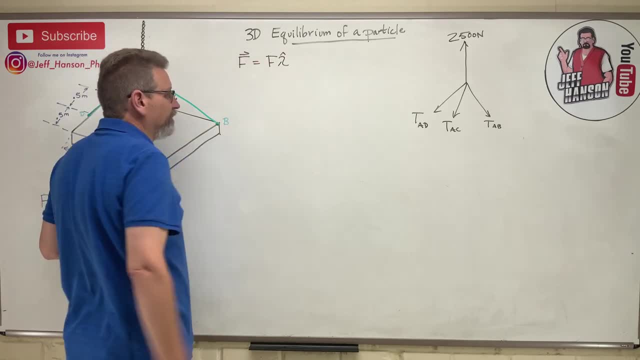 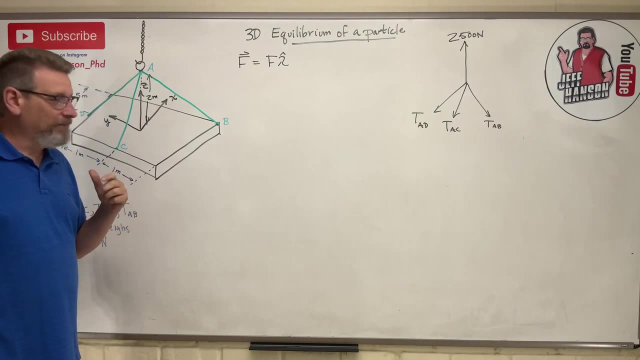 is equal to magnitude times direction. okay, now you're. typically students are going to get good at this because it's very repetitive. okay, we do it over and over and over. maybe by the 100th time we do it you start to catch on. this is a not a hard problem on the test, but this may be the 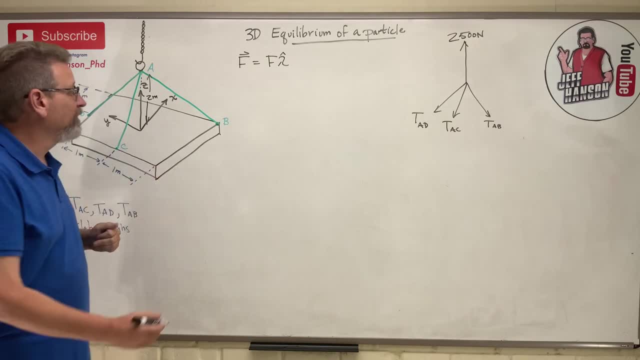 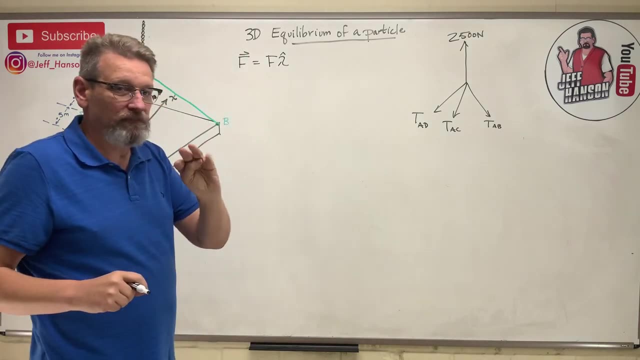 longest problem, just because of all these steps we have to go through. okay, so what we're trying to do is: we're trying we have how many ropes, what? two, three, four. I need to write all four in cartesian form, in IJK form. okay, so do that. 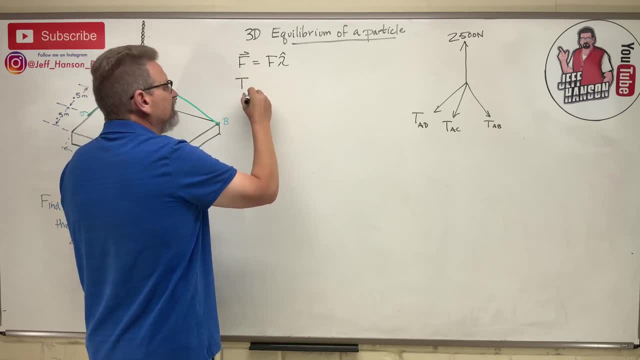 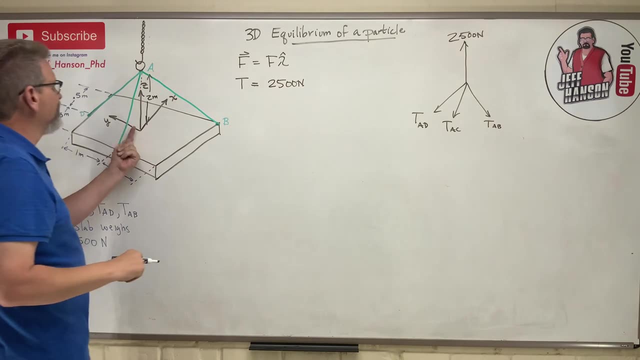 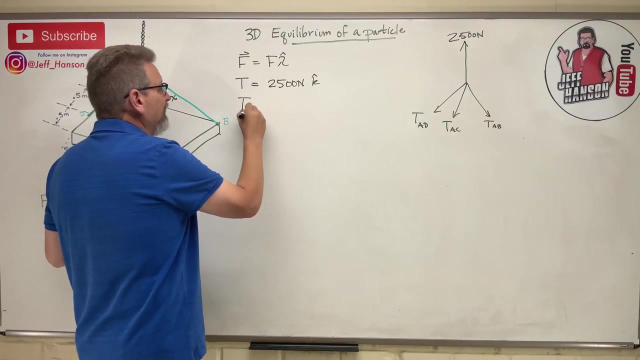 first one up there first. okay, I'm just going to call him t for tension. I don't know what he is, but he's. I'll tell you what he is. he's 2500 newtons in the. what direction is that? that's the z direction. so that's a k hat done, okay, there's one done now. I need vector t a b. I need vector t a c. 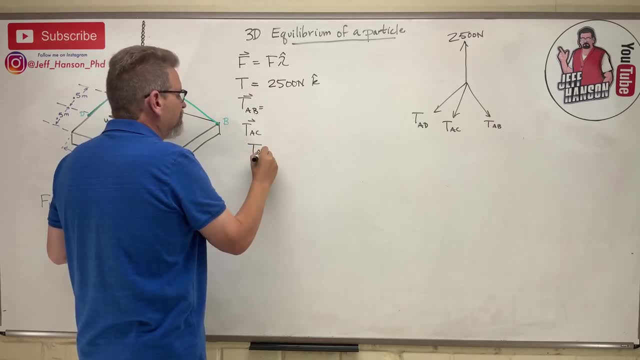 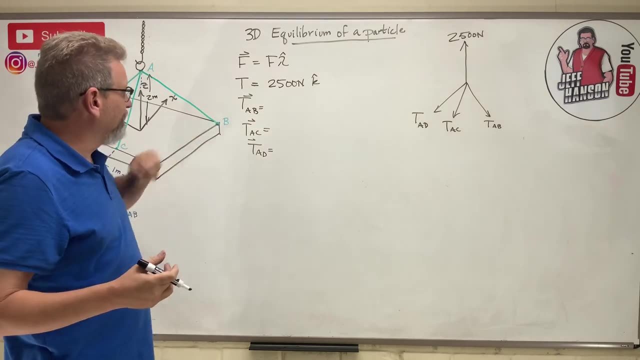 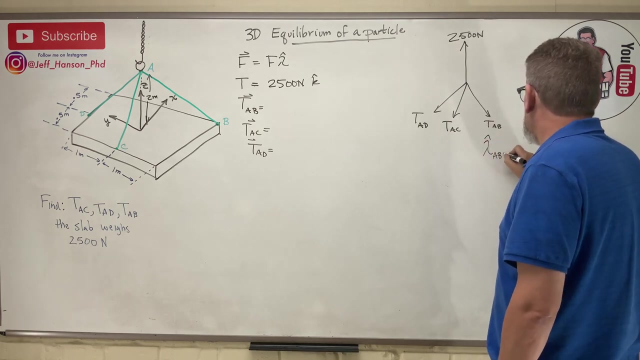 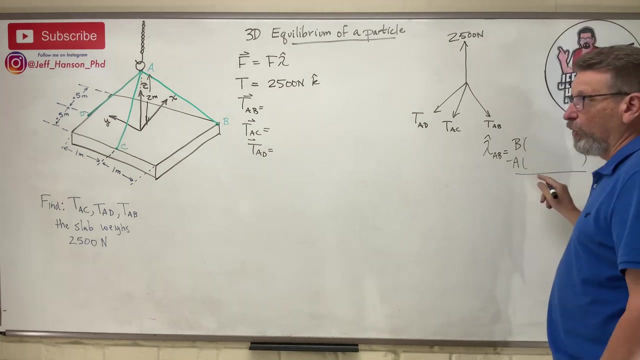 a little vector above them and I need vector t a d. okay, I need, I need all of those in IJK form. so let's just, let's just start with a b, okay, so here you go, lambda hat. a b is equal to b minus a. okay, so we need these coordinates now. the coordinate of point a is easy: it's zero zero two. 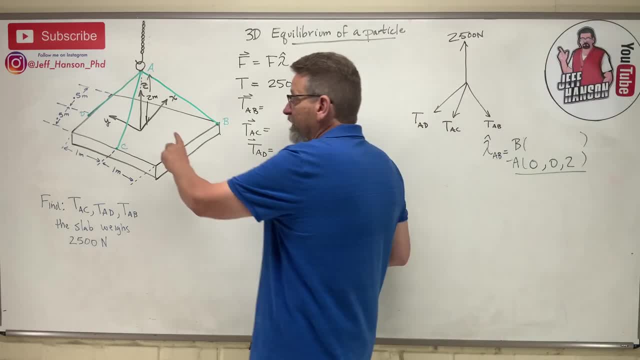 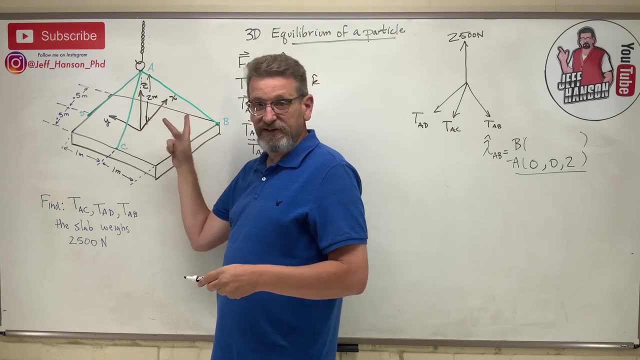 now, don't fall for this trick. look the. the coordinate system is kind of like spun around on us, right, so we're used to it being like this, but it's like that. it's the same thing. but just remember this is y and this is x, and remember where the positives are. okay. 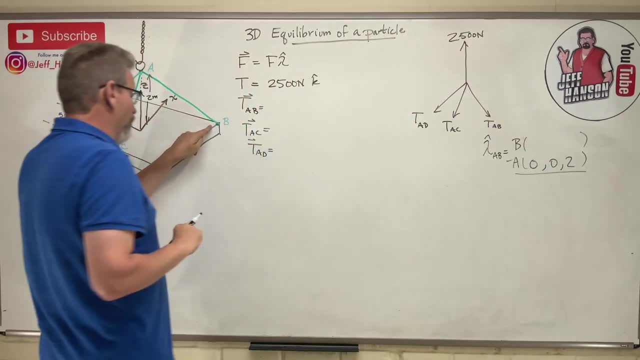 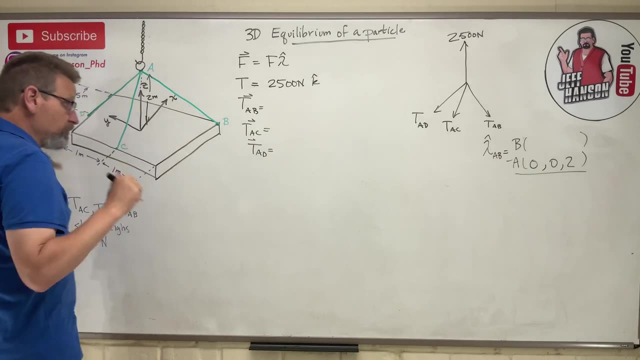 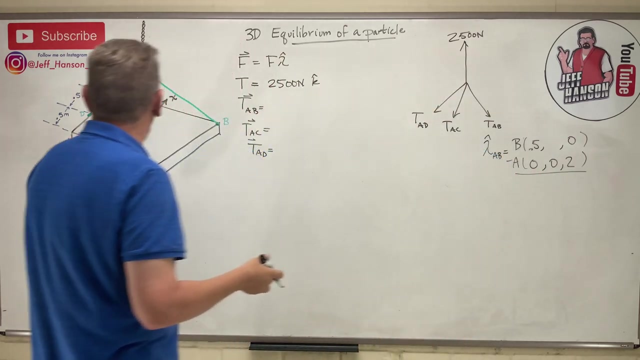 so what are the coordinates of point b over here on this corner? what are the coordinates on that corner over there? okay, in the x I have to go 0.5. whoop, so 0.5 in the x. I have to go 0 in the z, because no that that it's down on the plate right. and then how much in the y? 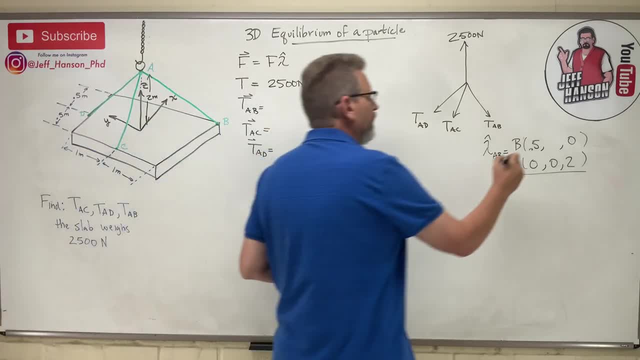 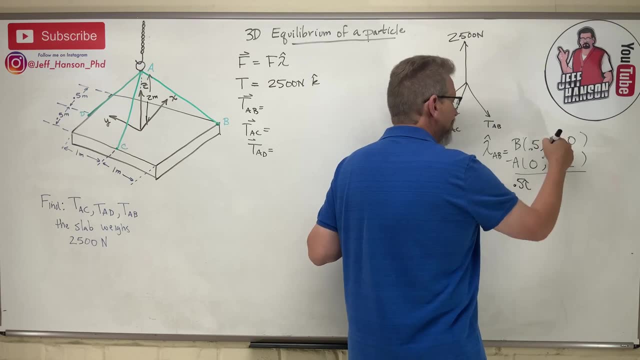 it's negative one, all right, negative one, okay. so here we go: 0.5 minus zero is 0.5, and then minus one minus zero is still minus one, and then zero minus two is minus two divided by the magnitude point five: 0.5 squared plus one squared plus two squared. let's see what that is. okay, wake up calculator. 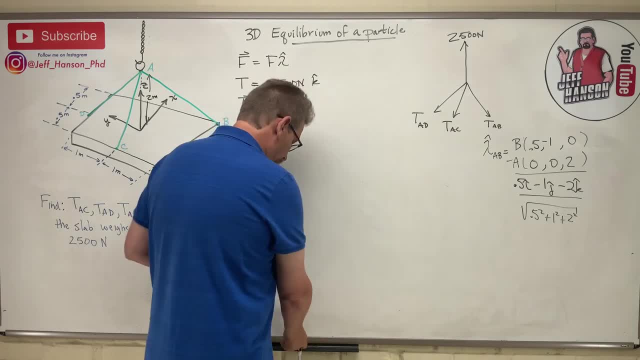 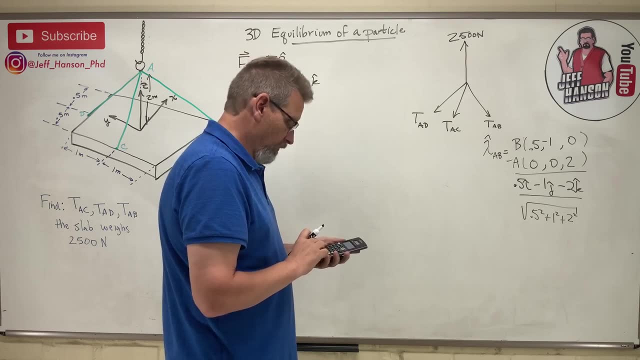 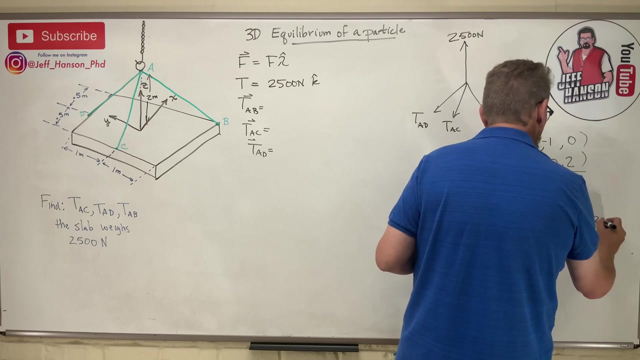 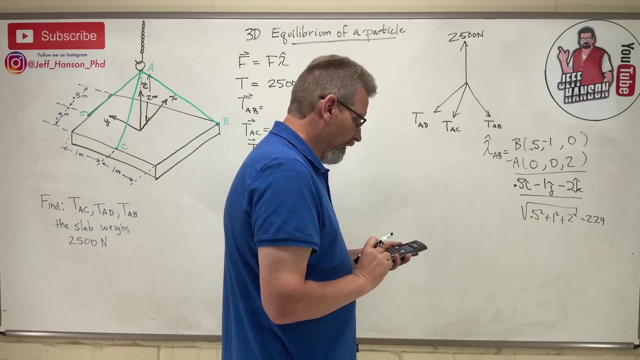 my calculator is sick, okay, I have to reset it every time. here we go: 0.5 squared plus one, plus four equals, and then undo, or second square root is 2.29. okay, so lambda hat a: b is 0.5 divided by 2.29 equals 0.218. 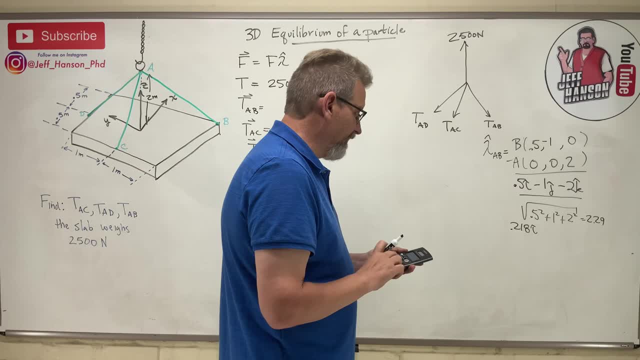 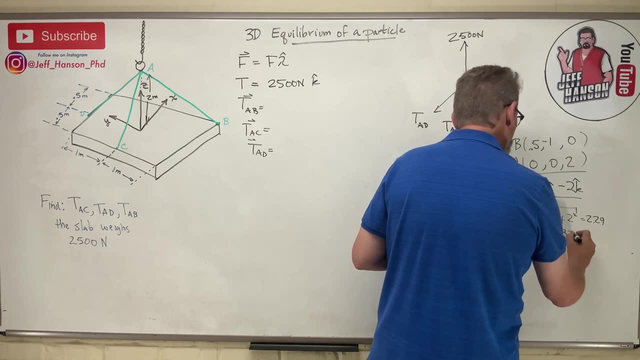 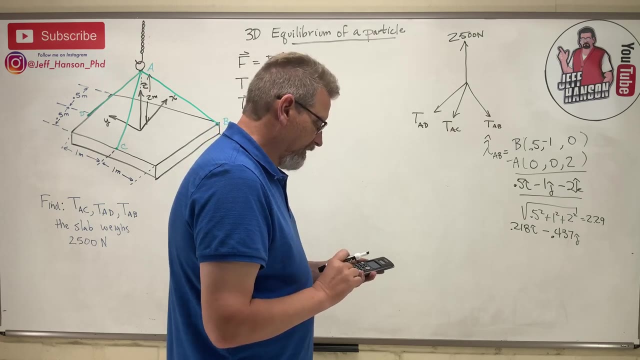 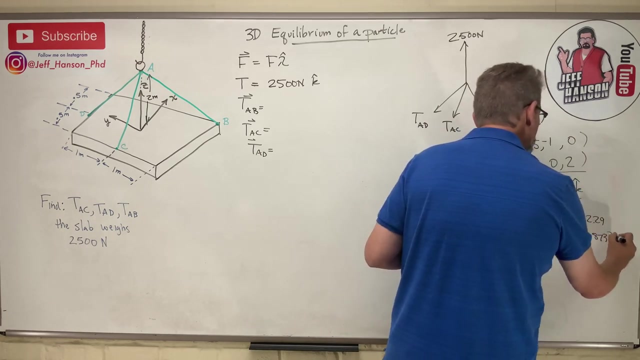 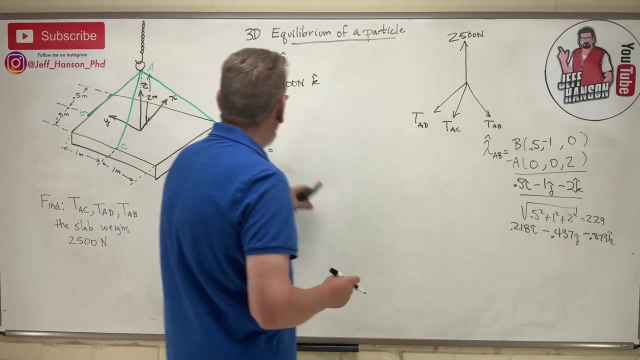 i hat, and then 1 divided by 2.29 is 0.437, j hat, and then 2 divided by 2.29 is 0.873. and remember, if this guy is positive, negative, negative, then this guy has to be positive, negative, negative. okay, so that's a, b, so we can say that it's tape which we don't know its magnitude. 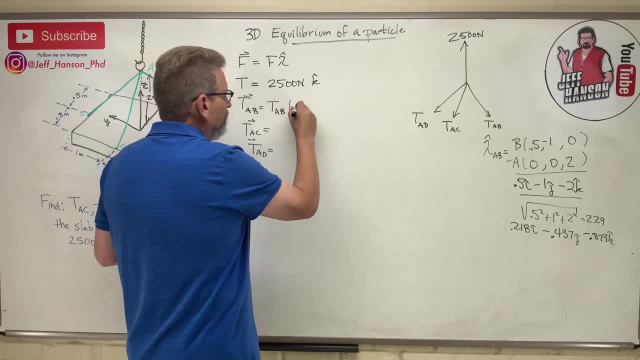 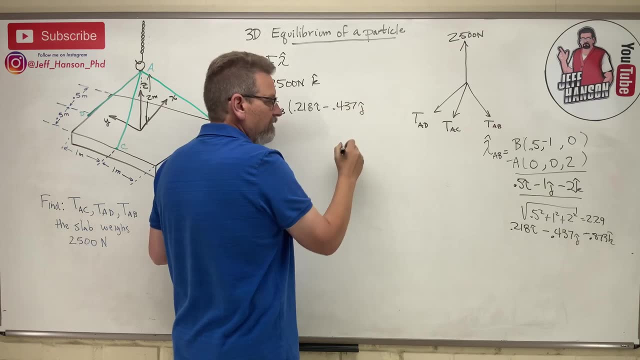 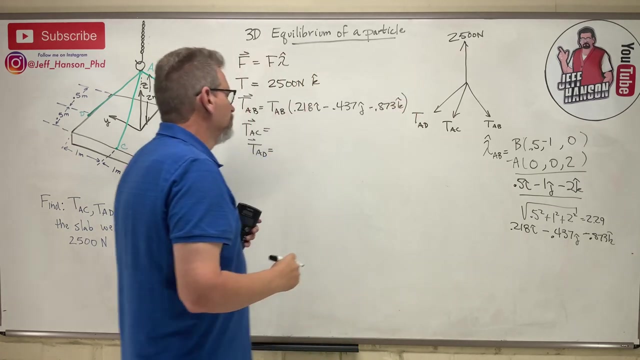 that's actually what we're looking for. times 0.2.. 2,, 1,, 8. I hat minus 0.437 J hat minus 0.873 K hat. Okay, There's one. Guess what we got to do. 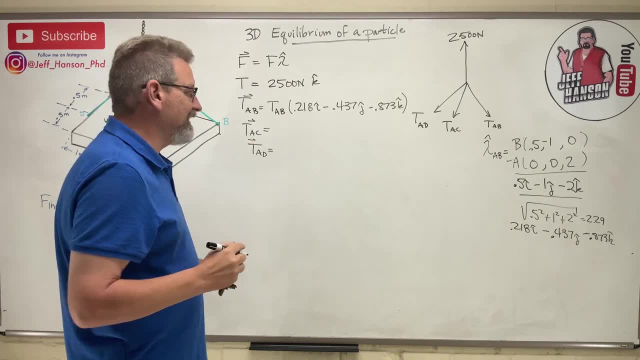 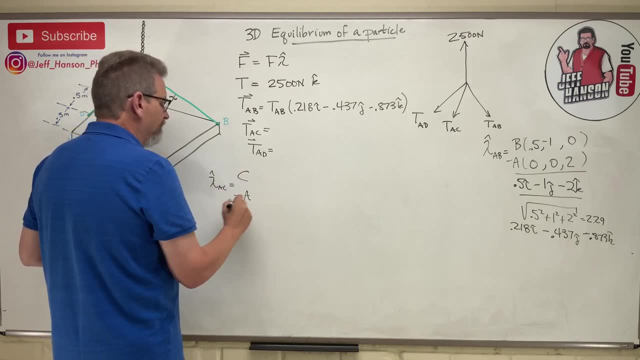 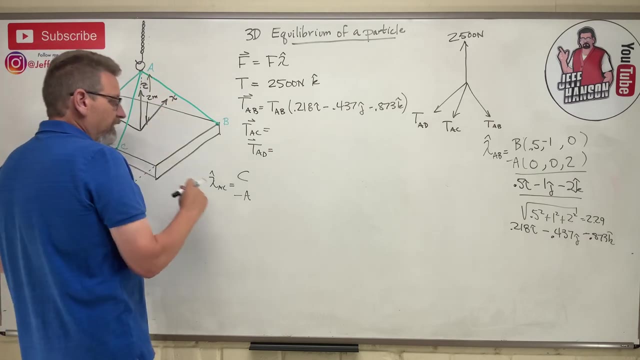 now Do it again. Okay, AC, Okay, Lambda hat. AC is C minus A, right, If it goes from A to C. right, The vectors go from A to C, Then we do A to C, is this way? Then we do C minus A. 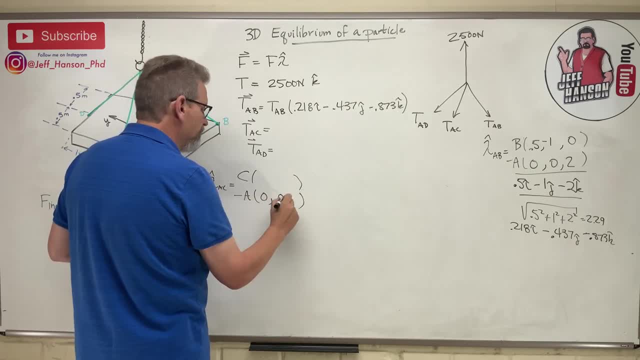 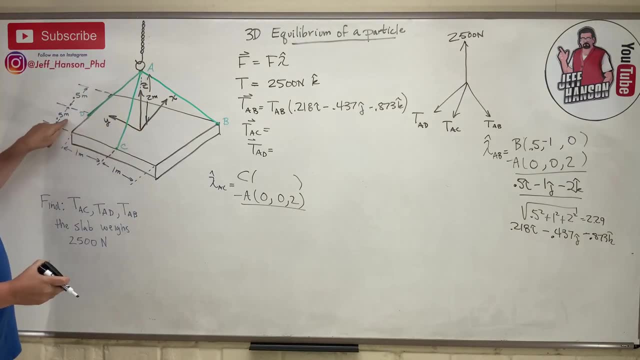 Now I already know what A is. We already got that guy. He's 0, 0, 2.. So what are the coordinates of point C? C is right here, So in the X I have to go negative 0.5,, negative 0.5. 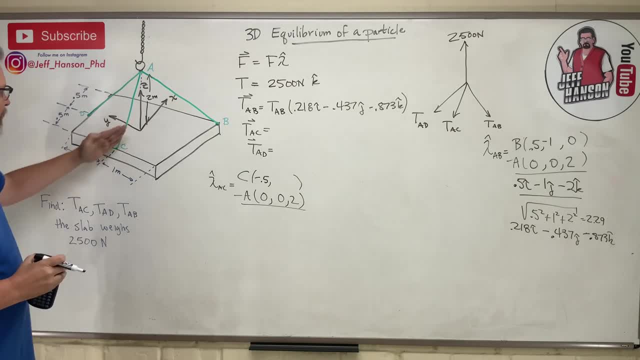 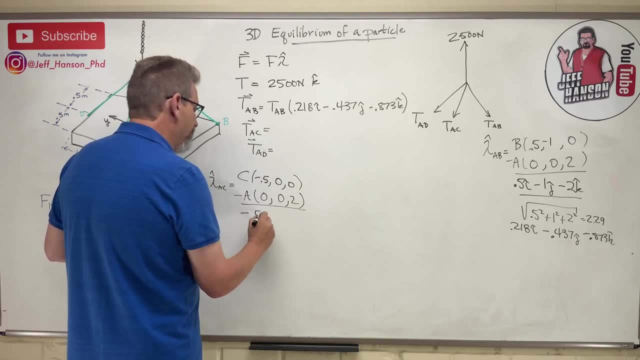 And in the Y I have to go: oh, 0.. It's right in the middle, isn't it 0, 0, and then 0 in the Z. Okay, So minus 0.5. I hat plus 0, J hat minus 2, K hat All right Divided. 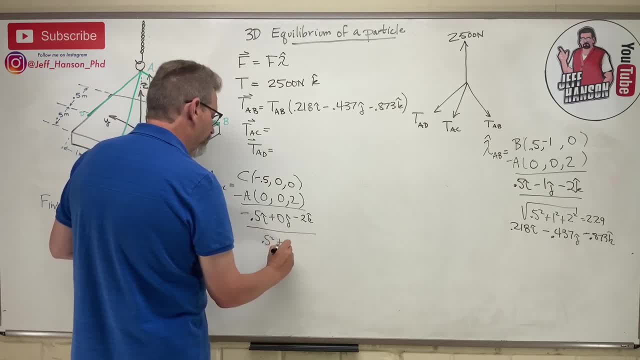 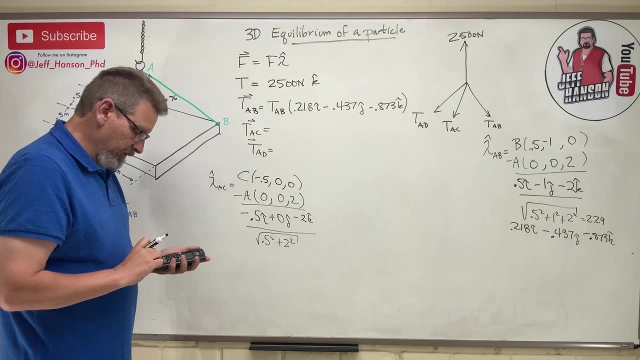 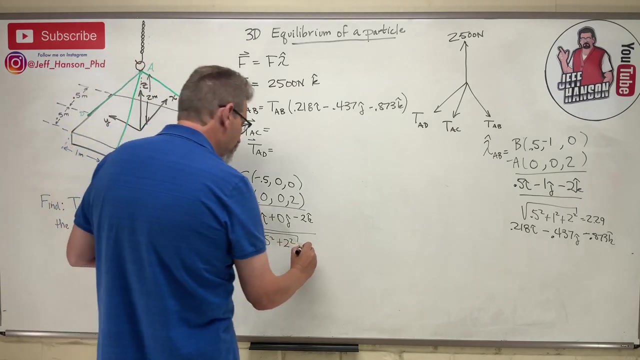 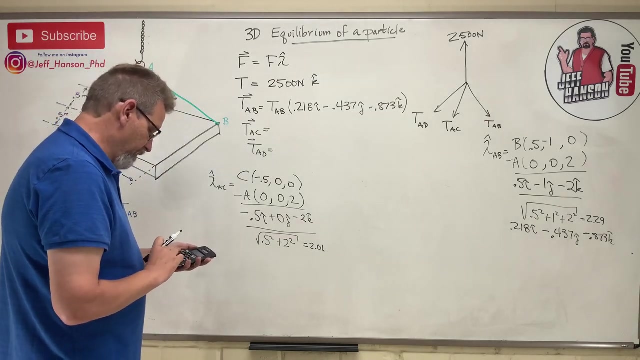 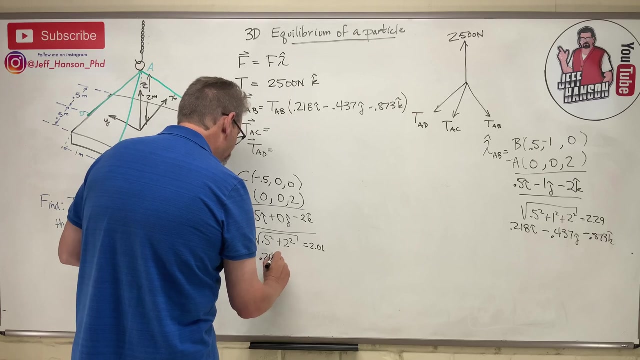 by 0.5 squared plus 2 squared square root. Okay, 0.5 squared plus 2 squared equals square root. Answer equals 2.06.. Okay, And so let's do this one. So 0.5 divided by 2.006, 0.248.. So 0.248 I hat. 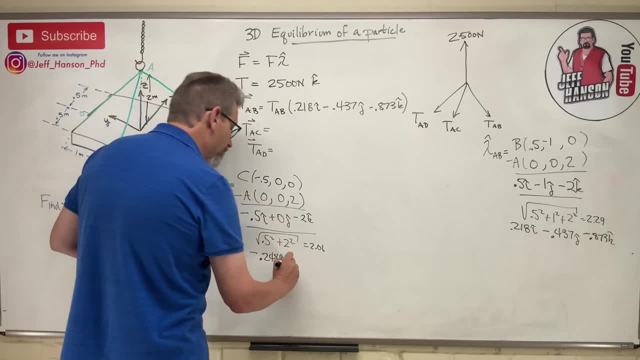 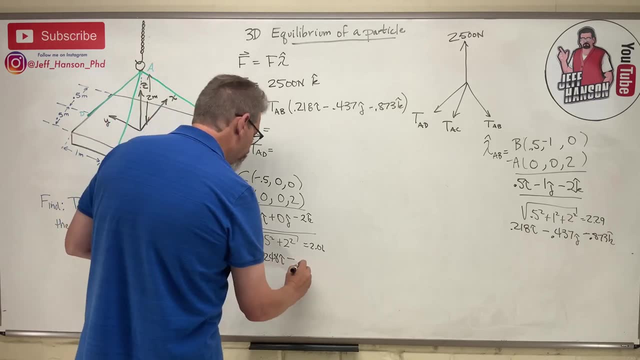 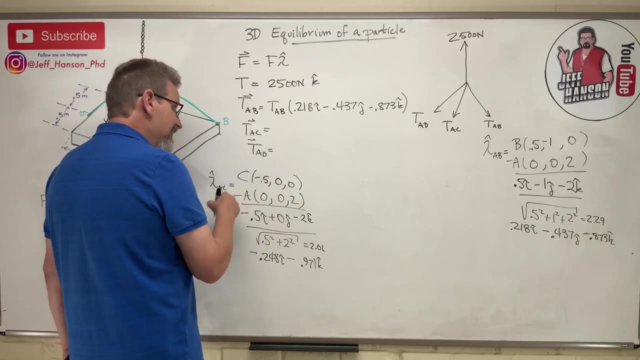 but that's going to be negative, right, And then negative. what's K hat going to be? 2 divided by 2.06, 0.971.. K hat- Okay, So that's going up here. That's T A C. So I don't know that one T A C times. 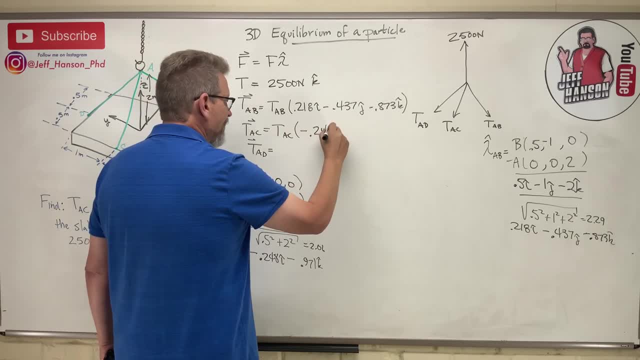 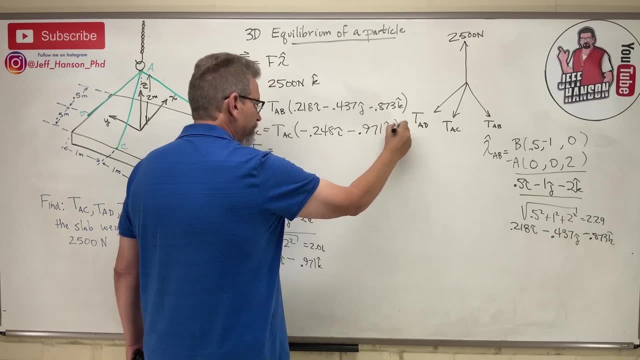 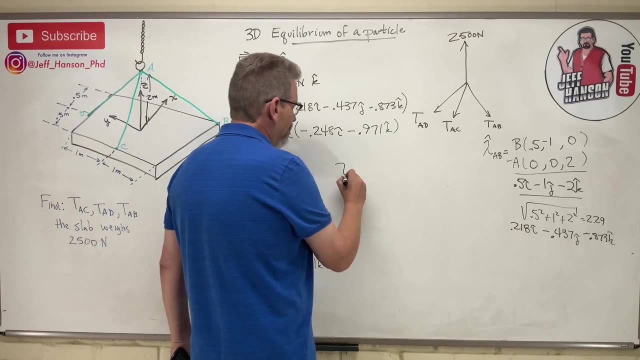 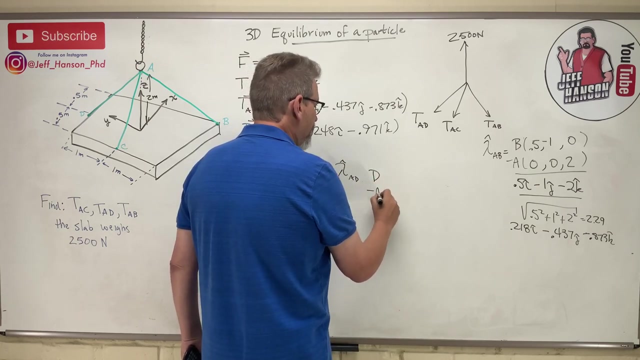 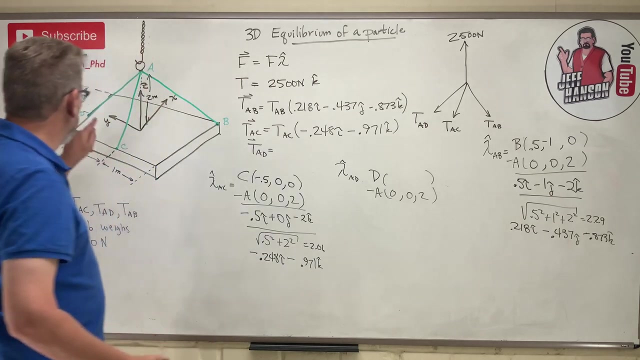 lambda hat, which is negative 0.248. I hat minus 0.971 K hat. Okay, One more game And that is A D. Okay, How do you find A D Lambda hat? A D is equal to D minus A. Okay, I already know, A is 0, 0, 2.. So what is D? What is D? How much in the X? 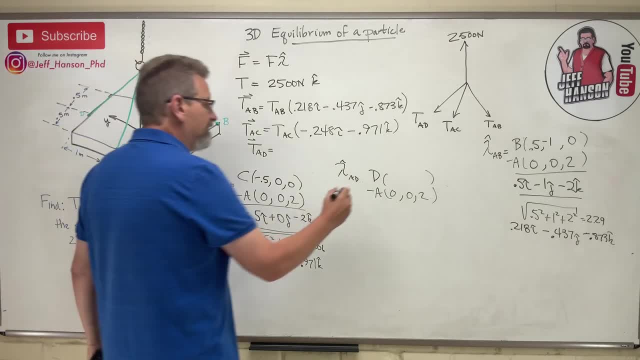 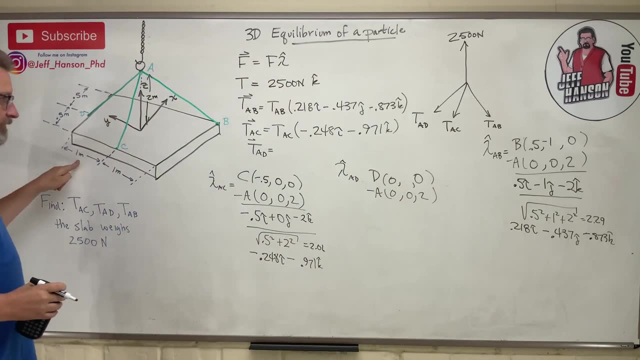 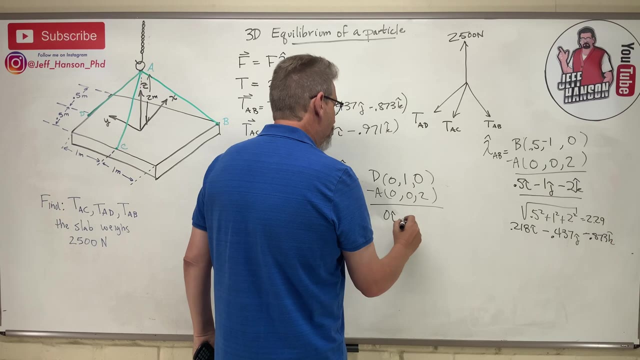 Zero Right, Zero in the X, Zero in the Z And how much in the Y? A positive 1.. Okay, So here we go. So I get zero K hat, 1 minus 0 plus 1 J hat and then 0 minus 2.. 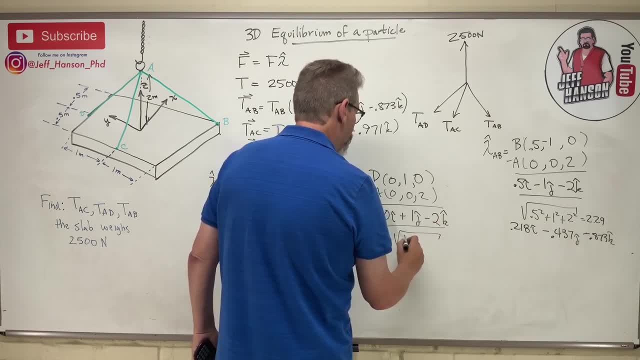 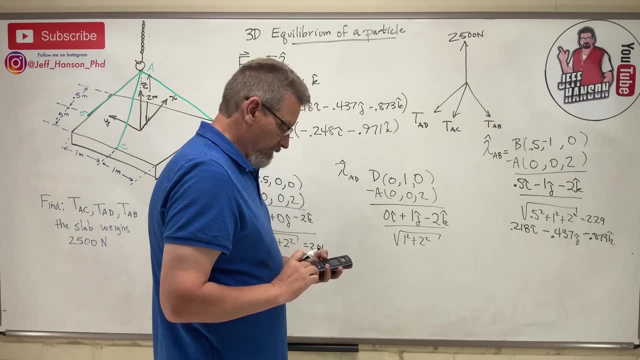 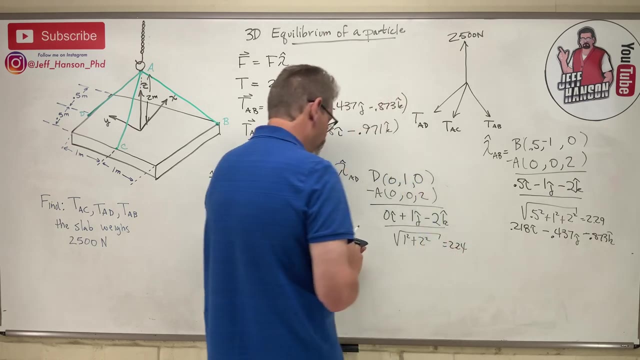 Okay, Divided by square root of 1 squared plus 2 squared, What is the square root of 5? The square root of 5 is 2.24.. And so that's 1 divided by that is 0.447.. 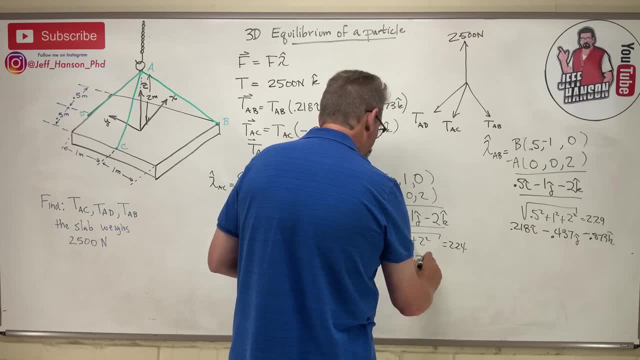 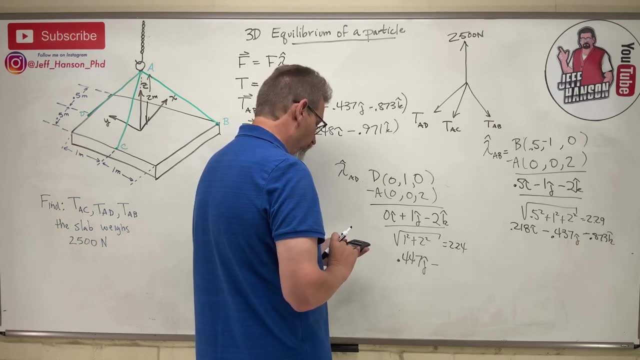 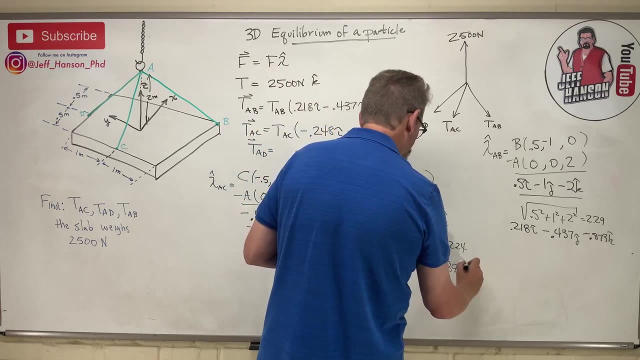 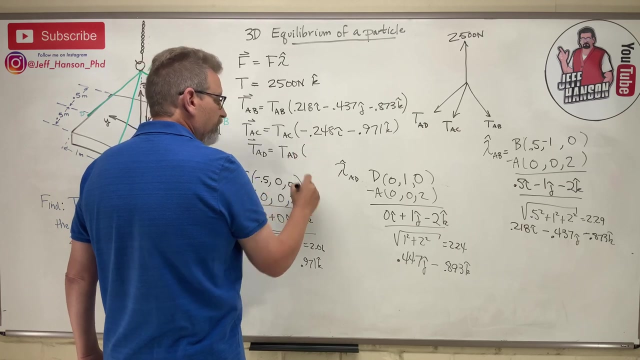 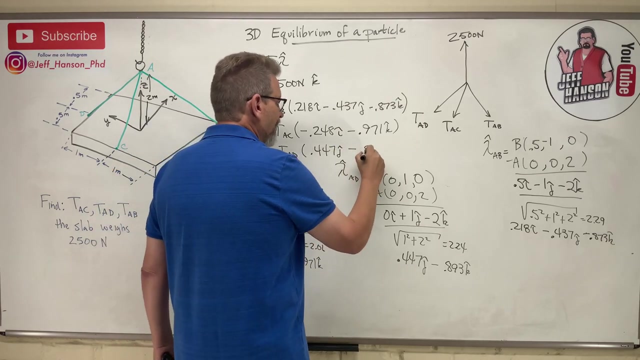 And that's positive, And then minus 2 divided by 2.24.. 0.893.. Okay, And so there's my last vector, T A D. It's going to be 0.447 J hat Minus 0.893 K hat. 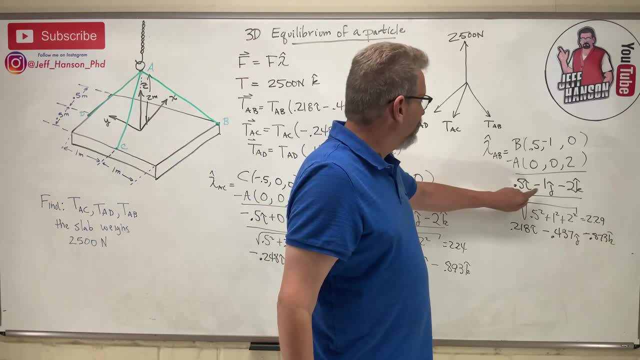 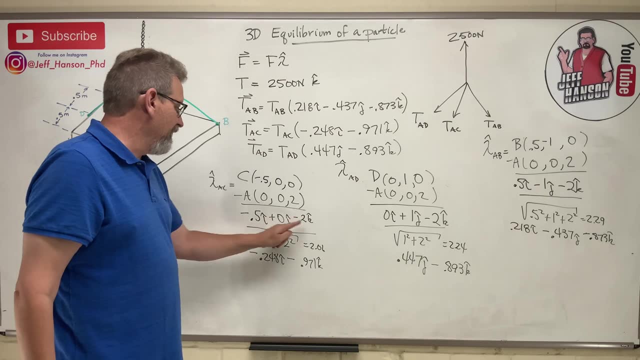 Now just make sure you get your signs right, right, Positive, negative, negative, Positive, negative, negative, Positive, negative, Positive, negative, Negative, negative, negative, negative. Okay, I feel good about that right. So easy to do. I do it all the time. You got to be careful. 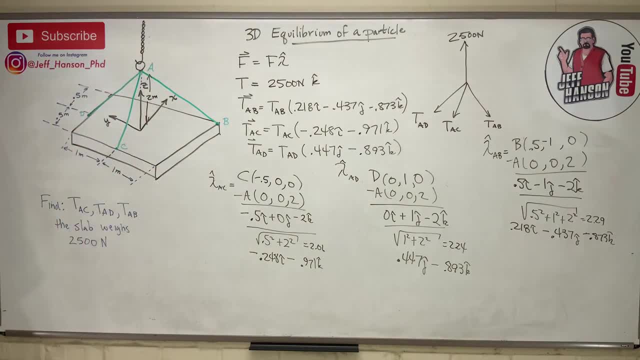 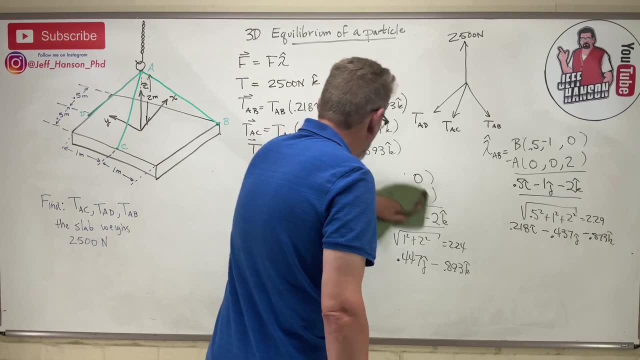 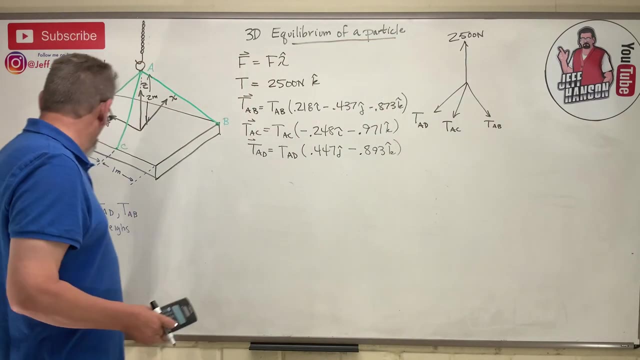 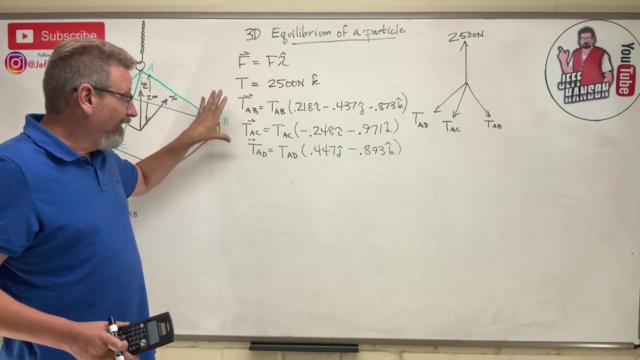 Let's erase some of this. Okay, Here we go. So we're about halfway there, maybe a little more, because now we have all our vectors written in IJK form, in Cartesian form. All we need to do now is build what I call the equations of equilibrium. 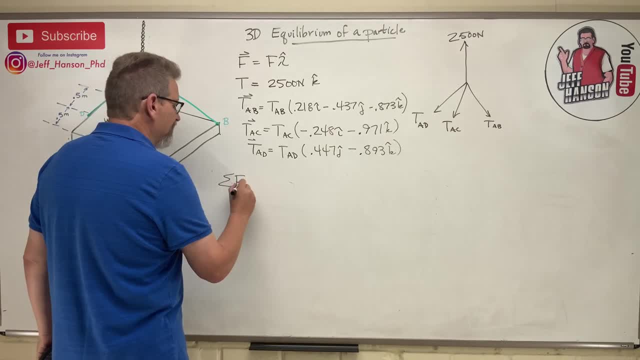 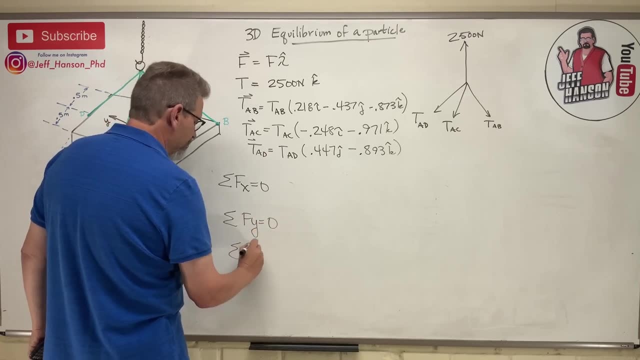 Okay, And they go like this: Some of the forces in the X got to equal 0.. Forces in the Y And some of the forces in the Y got to equal 0. And some of the forces in the Z. Okay. 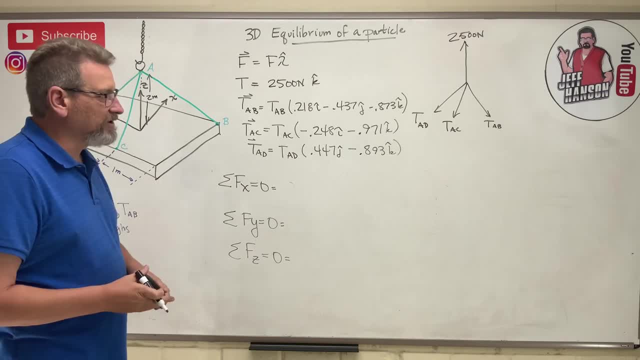 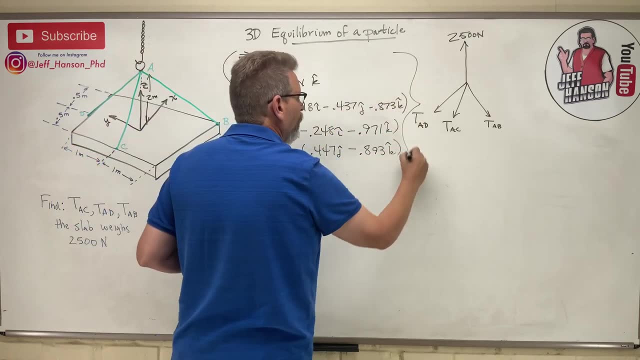 Now, how hard is it going to be to fill in these equations? Well, here's all the stuff that goes in these equations, right here, Okay, So how do I know what to put where? Well, guess what goes in the X equation. 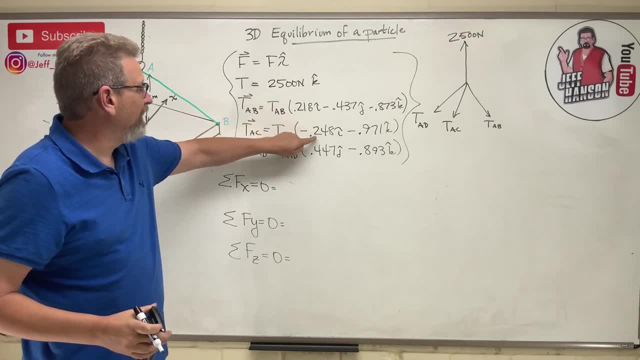 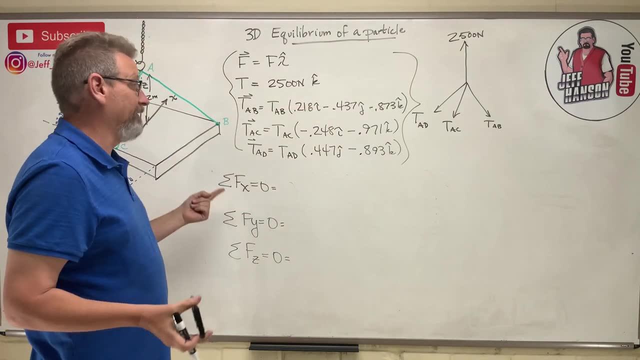 Everything that has an I hat on it, Okay. So U and U Who goes in the Y equation, Everything that has a J hat. So U and U Who goes in the Z equation, The K hat right. So let's just build these equations real quick. 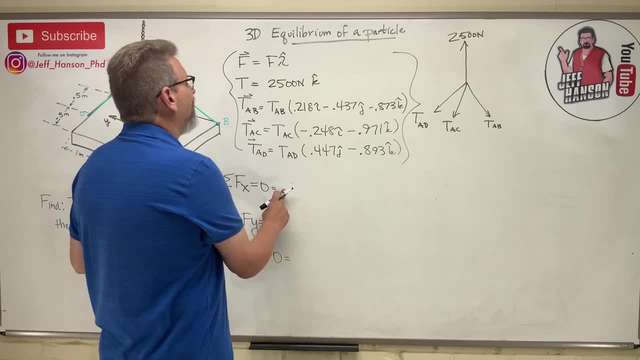 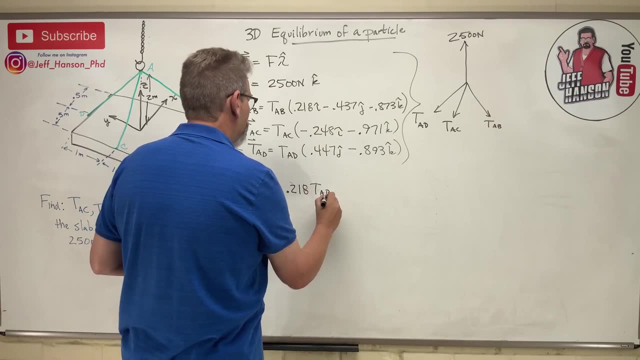 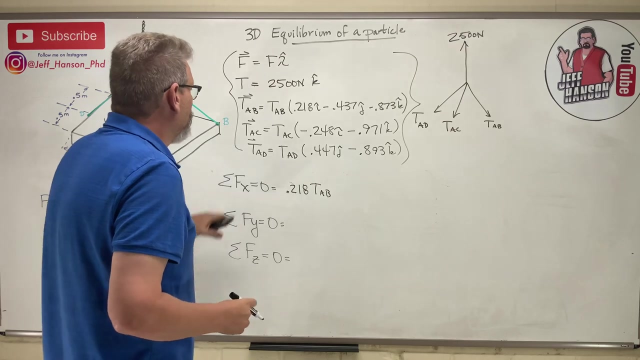 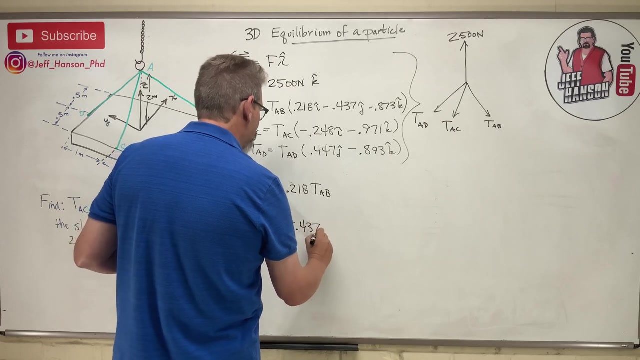 Okay, And we get. what do we get here? So in the I hat we have 0.218 TAB. Okay, And again, I'm going to be very careful and keep all this tabulated in the correct columns. Okay, So in the Y for TAB is negative 0.437 TAB. 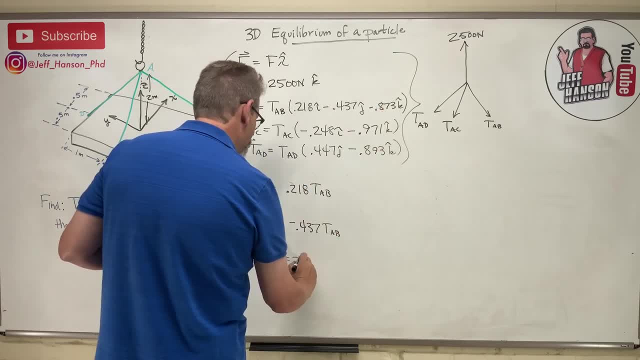 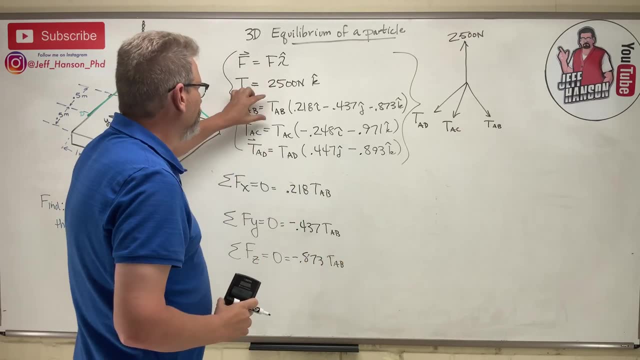 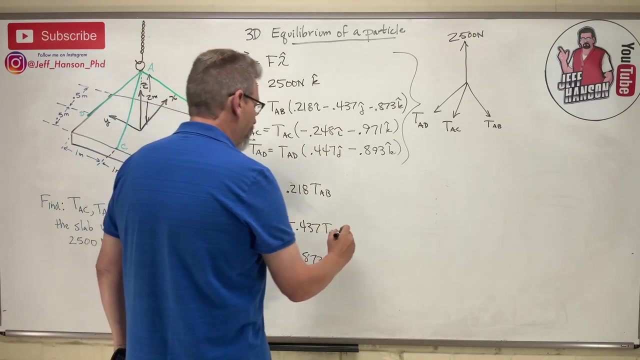 And in the K is negative 0.873 TAB. So there's all the TABs. right Done, Let's go to this guy, TAC. He just has an I and a K. He has no J. You know, I'm going to still put him in there, though, right? 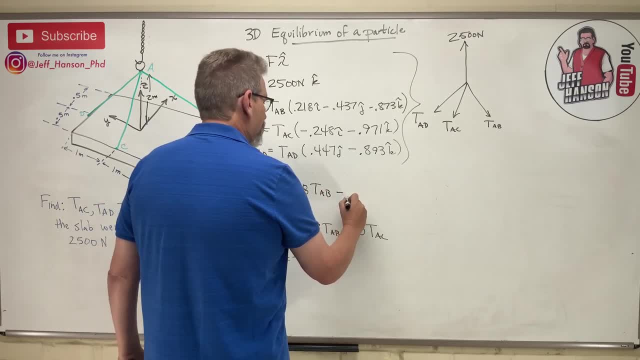 I'm going to put plus 0 TAC- right, He's just there, but he's not really there- And then minus 0.248 TAC. D right TAC: 0.248 TAC. That's a negative, that's a negative. 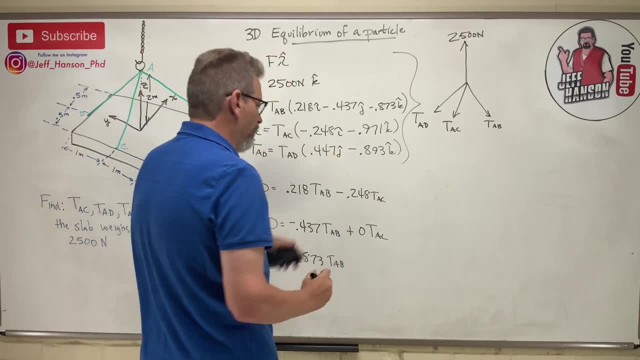 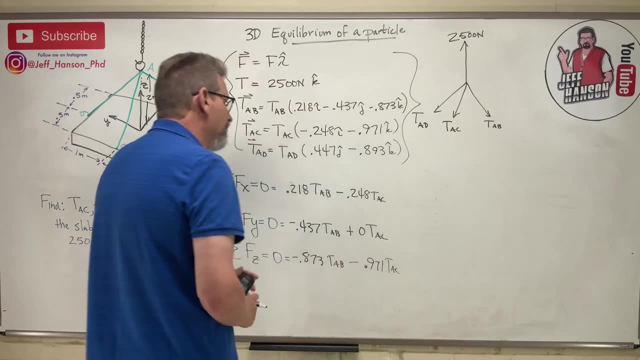 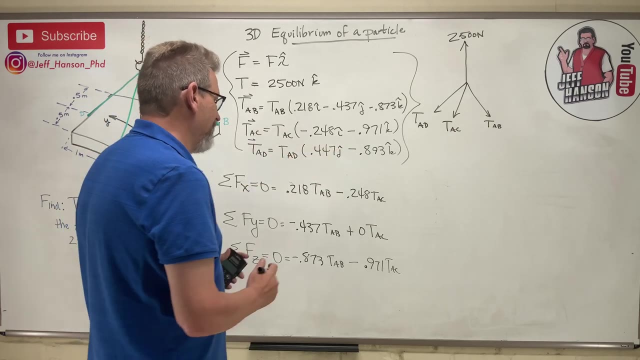 All right, So I'm going to put it in there. I'm going to put it in there, and then this guy here also minus right, minus 0.971 TAC. okay, so, there's that one done, there's that one done and we're on TAD. he's got a zero in the I and he's got a J and a K. 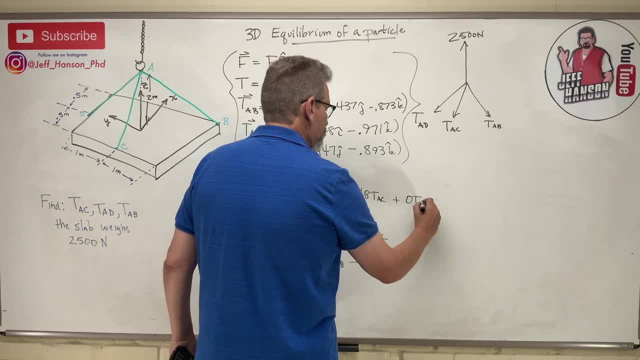 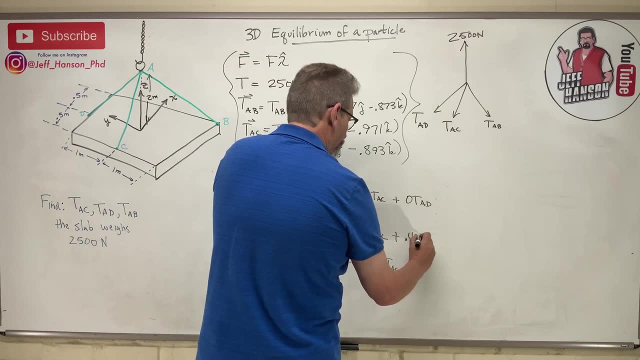 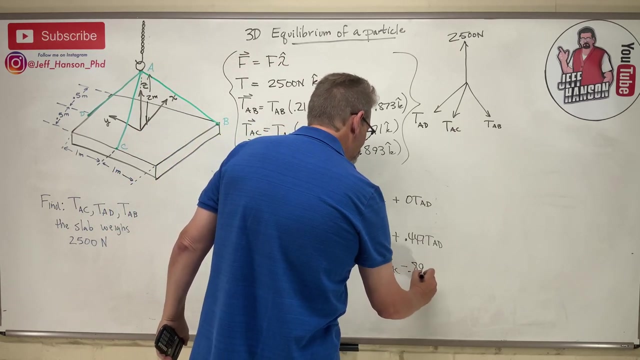 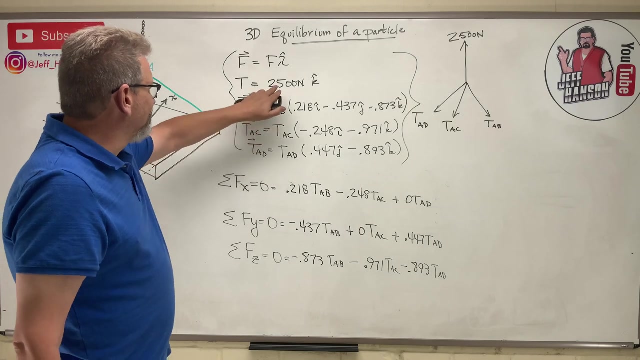 so plus 0 TAD- okay, plus 0.447 TAD, and then minus 0.893 TAD- okay. and there's one more, and that's this guy, and he's going positive in the K hat now look. 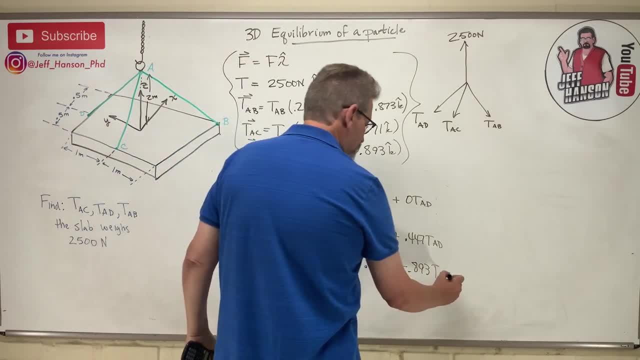 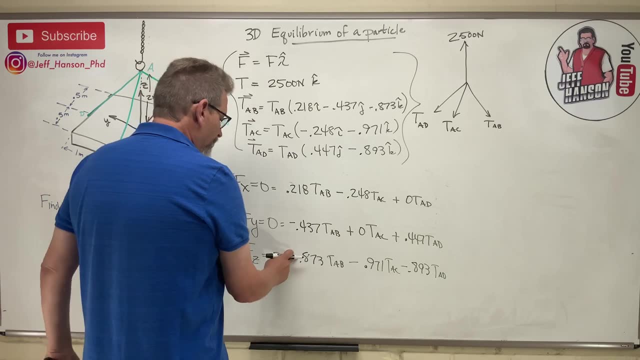 negative, negative, negative and then a positive right. so plus 2,500,. well, what if I left the 2,500 there and then moved all of those negatives to the other side? well, they would all change to. 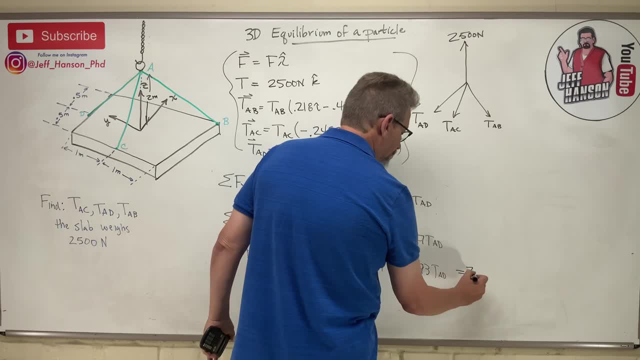 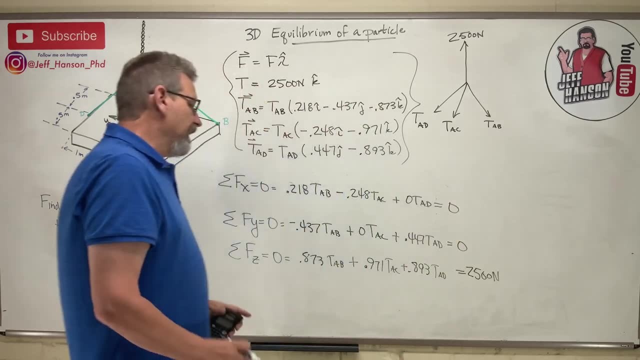 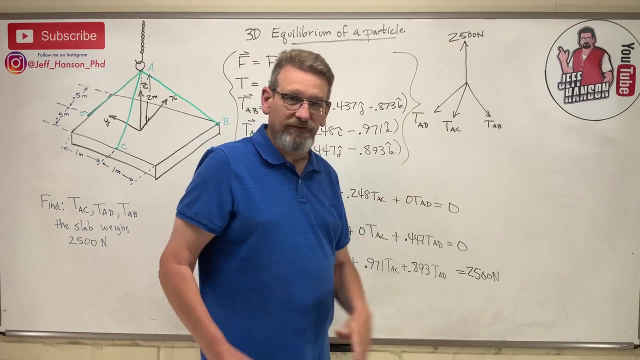 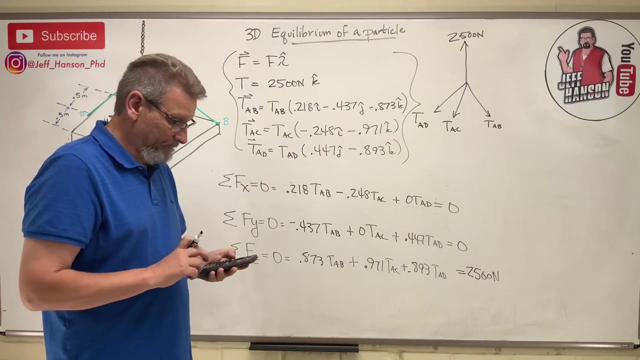 positives equals 2,500 newtons. okay, equals zero equals zero. now look what I have here. okay, I have all my ABs, all my ACs, all my ADs and all my constants, perfect setup to use my system solver on my calculator TI-36 Pro. yo, what's up? here we go. 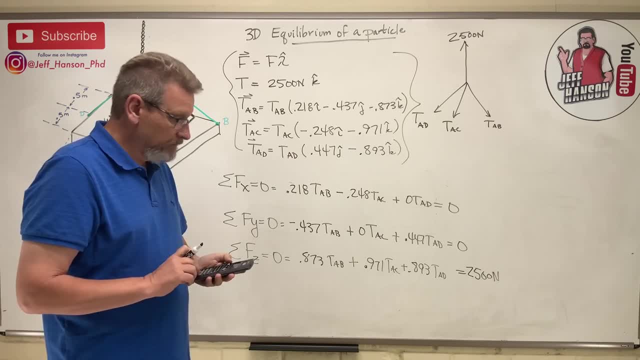 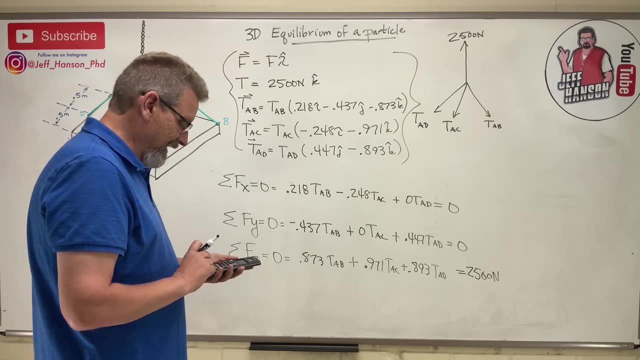 system solver. three by three enter. all right, I'm gonna put these numbers in real fast: 0.218,- whoa, that's not right. 218, enter and then negative. 0.248, enter and then zero enter.